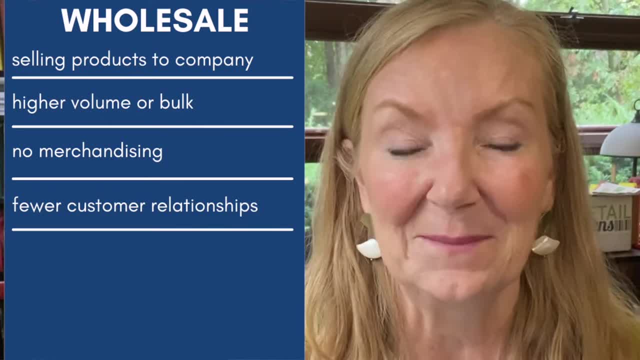 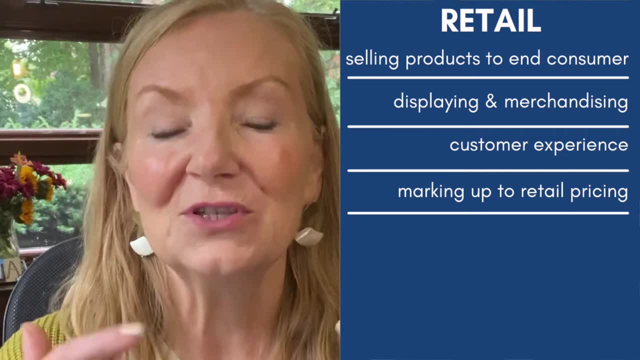 thing, but you don't have to manage as many customers at the same time, because you're selling to fewer people, but selling more items to those people. When selling products at retail, you mark the product up to the retail price. That then allows you enough gross margin to cover all the. 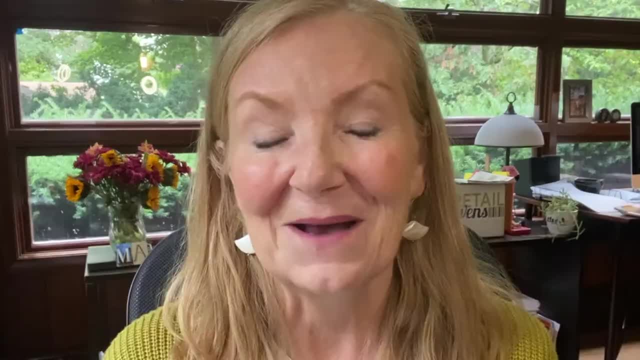 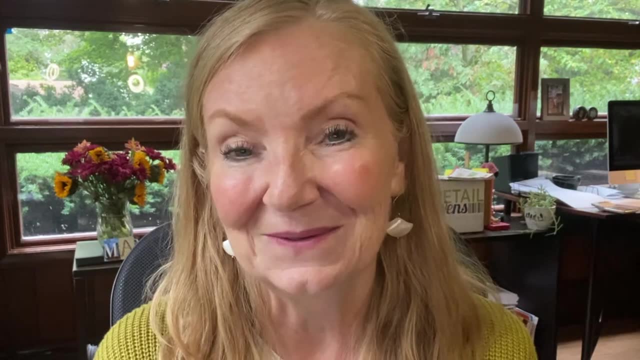 other expenses in the store. If you need more information about how to price your products for retail, including the percentage, you should mark your products up, which is also called an initial markup or IMU. stay tuned, I'm going to share more about that in just a bit. Pricing wholesale. 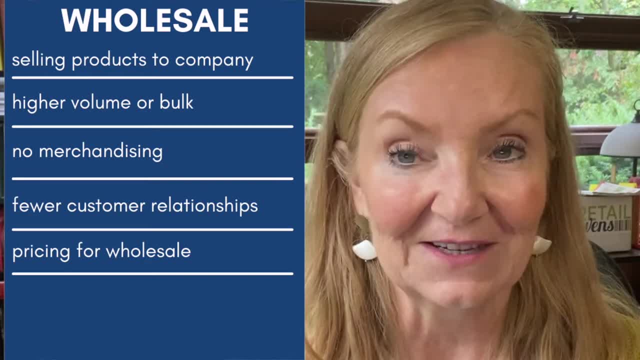 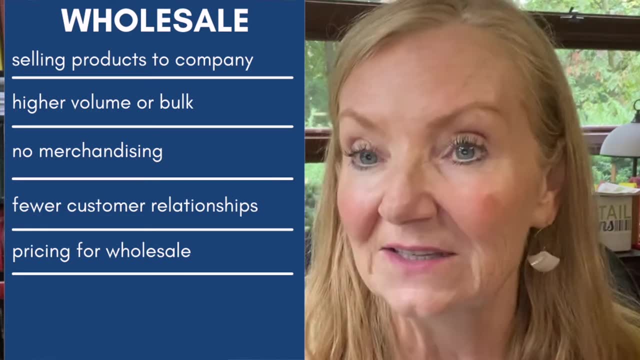 sales tax is different. It involves calculating your cost of manufacturing or buying the product. if you're buying it from another manufacturer and then marking it up to allow for profit for you as you sell to the retailer, The markup won't be as high in this case because your costs are all. 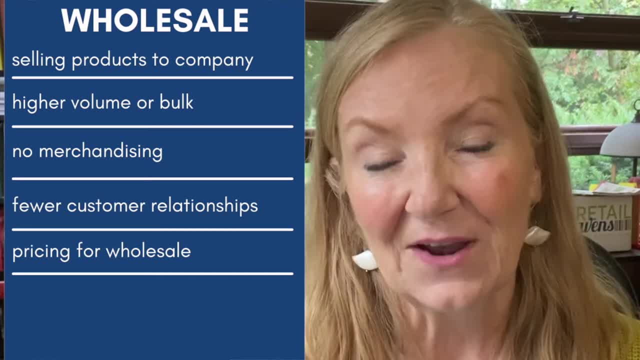 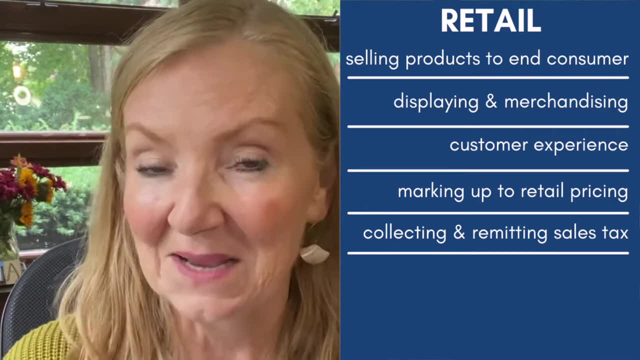 accounted for in the cost of the item, whereas a retailer has to also account for the cost of doing business. Sales tax is handled differently between the two. As a retailer, depending on where you live, you're usually responsible for collecting and remitting the cost of the item. If you're a 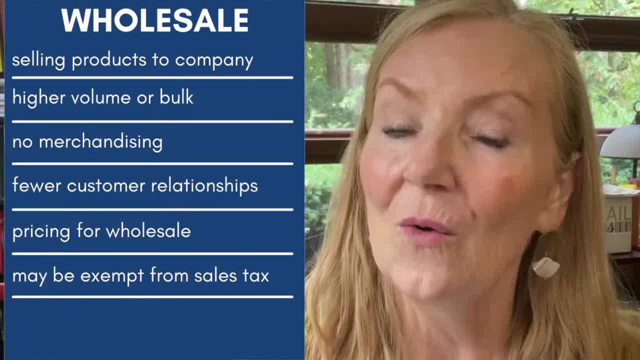 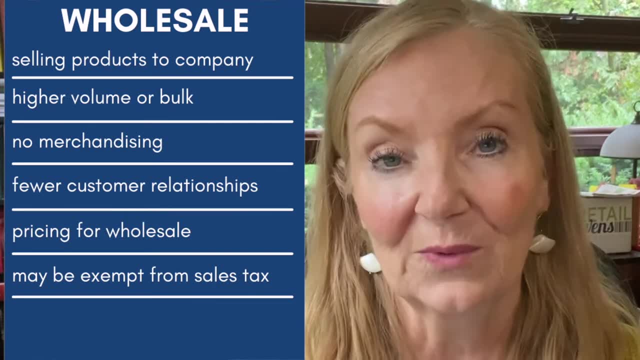 retailer, you're responsible for collecting and remitting the sales tax to the states that you do business in, whereas a wholesale businesses are usually exempt from collecting and remitting sales tax. You usually don't have to do that, but of course check with your local regulations. 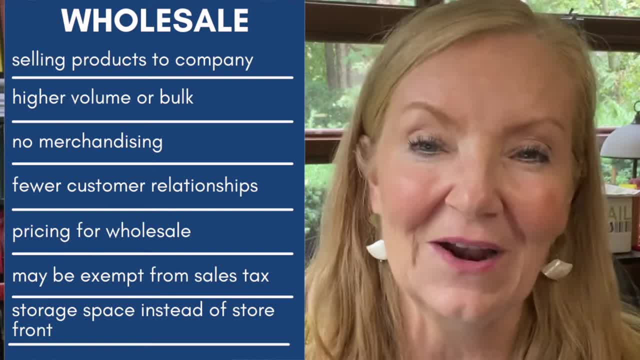 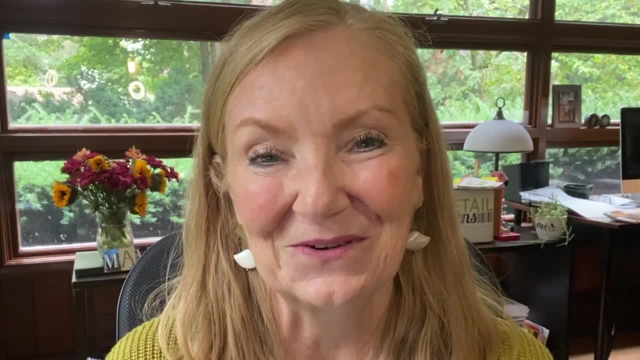 Wholesale doesn't require a storefront, but usually requires a warehouse or some sort of storage space for to hold the product in. A brick and mortar retail store does, by definition, require a storefront, but there also are many retailers now that are simply selling online also, so they 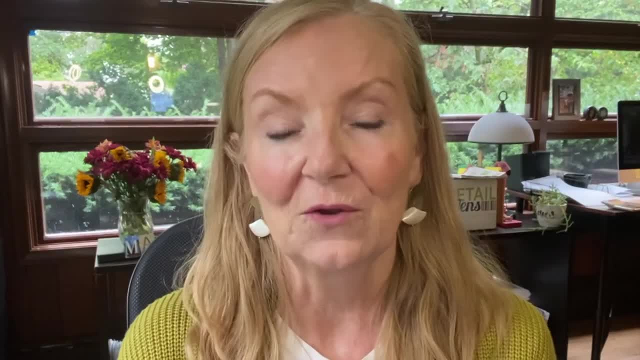 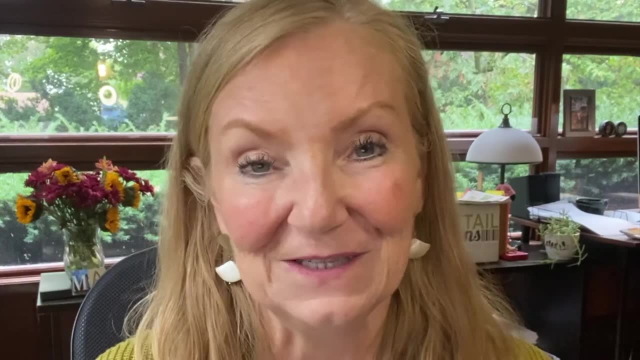 also require warehouse or storage space too. In both retail and wholesale, you have to communicate the features, the advantages and the benefits of the product to the buyer and, using a multitude of different platforms, to do that- The one other thing that retail does. 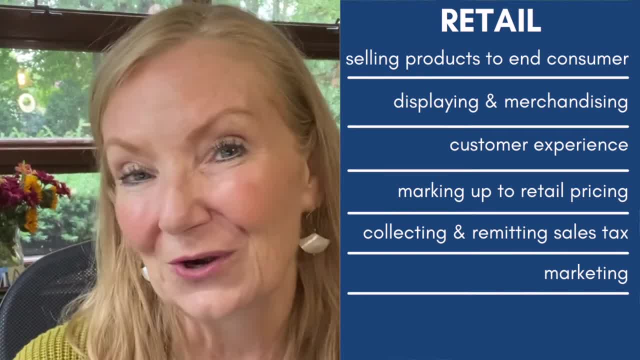 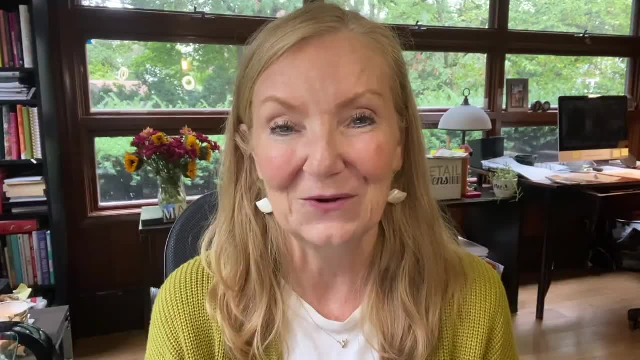 is that you're also talking about your store, the messaging of your store, but really also wholesale does the same thing. You should have a clear voice, a clear message that you're trying to get across for your wholesale company too. Another key difference is that wholesale usually